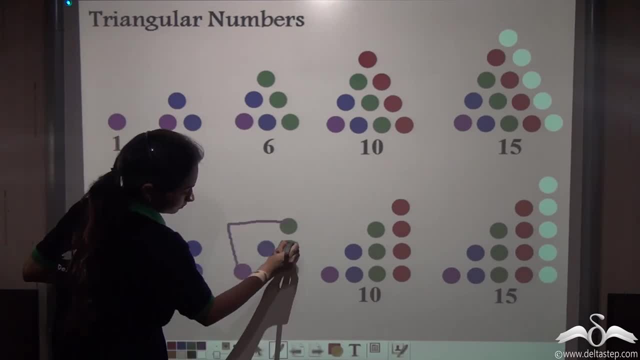 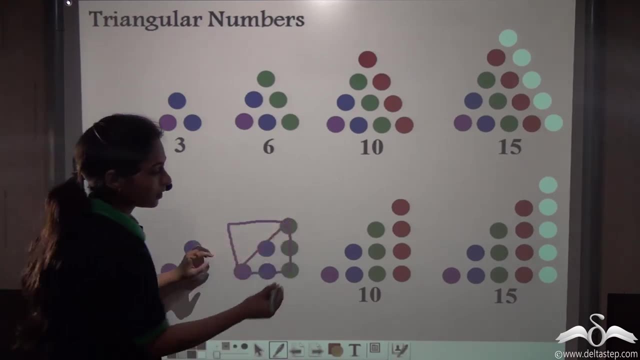 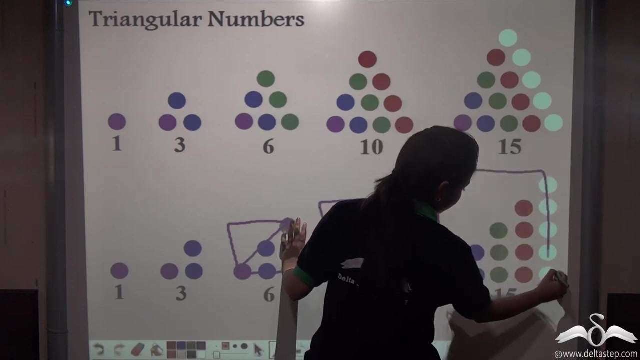 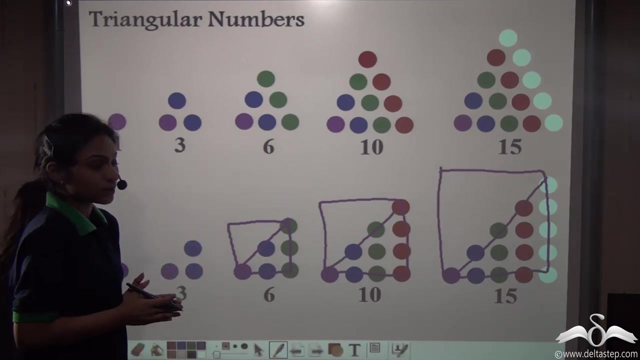 I am drawing this as a square. This is half of a square, isn't it? Doesn't it represent like half of a square filled with dots? Similarly, look at this and look at this, And adding any two of these consecutive triangular numbers, we get a square. So a square will. 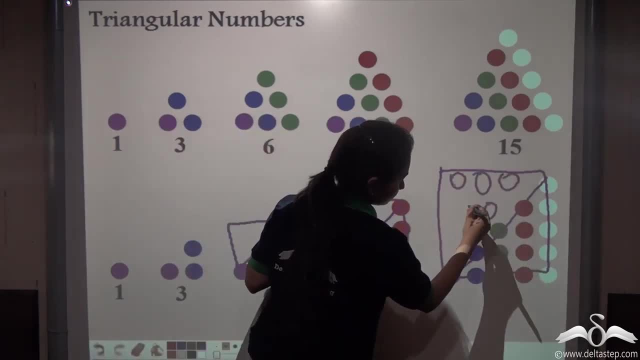 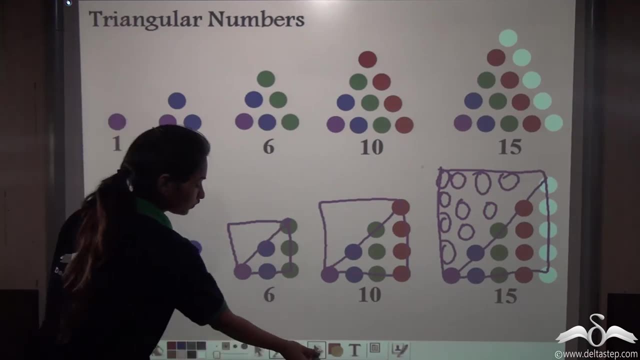 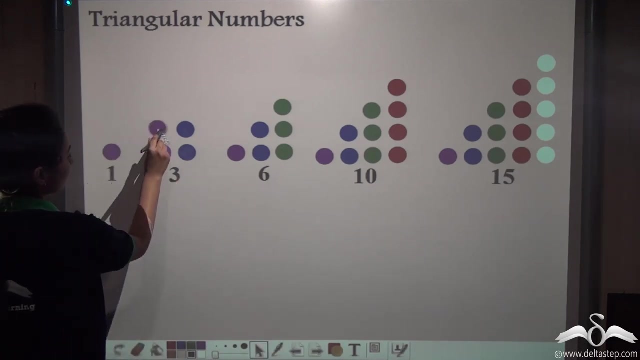 be what? Something like this. Well, does this happen? I will show you. First of all, adding 1 and 3. Add this 1 with 3.. See, you get a perfect square. Yes, Don't forget the point. 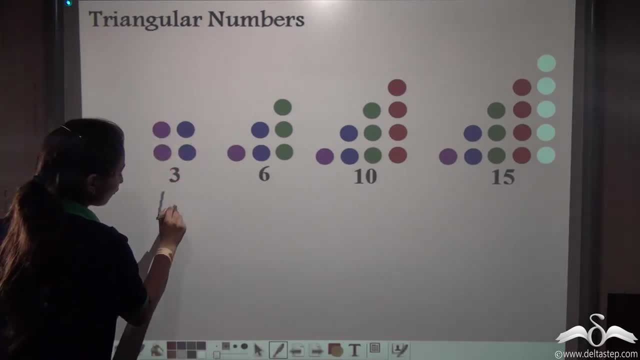 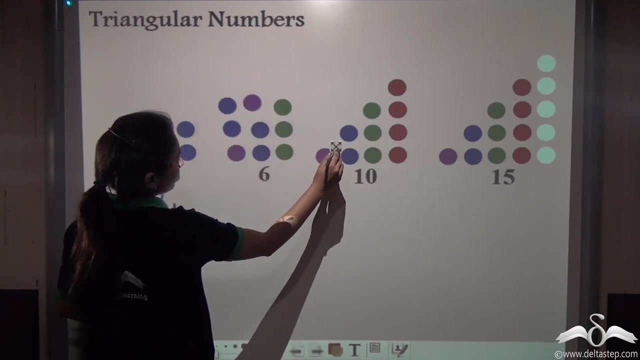 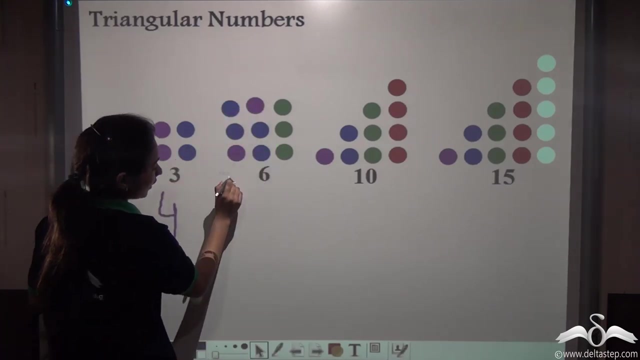 End of Ritual square. This is how you get 4. Now adding 3 and 6. Rotate it and add it. See what do you get: Again a perfect square. So I can say: 3 plus 6 gives me 9. That is a perfect square. 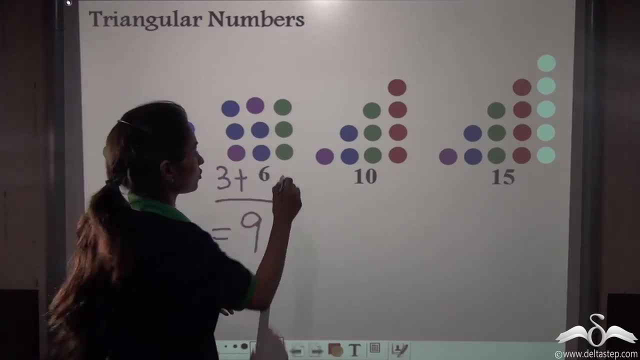 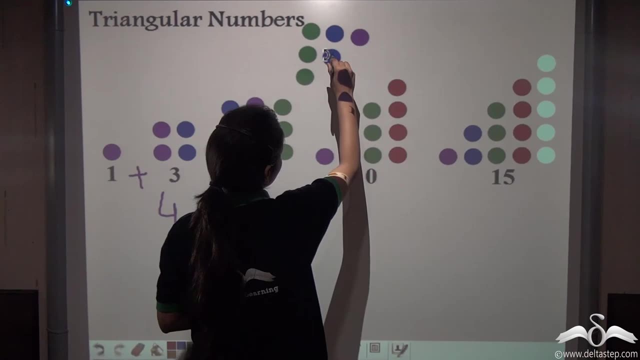 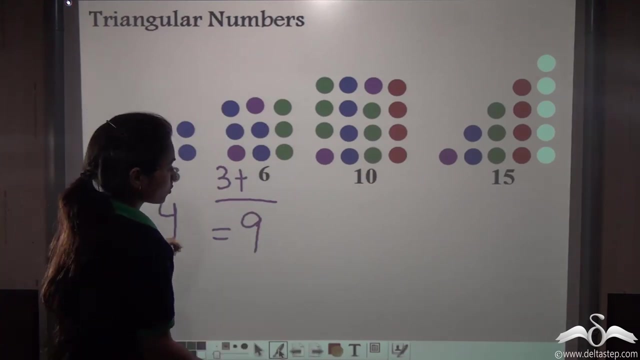 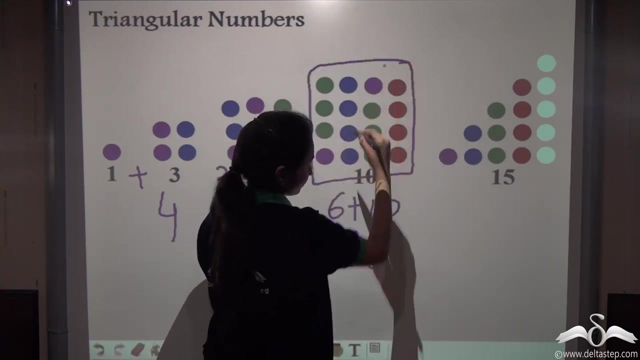 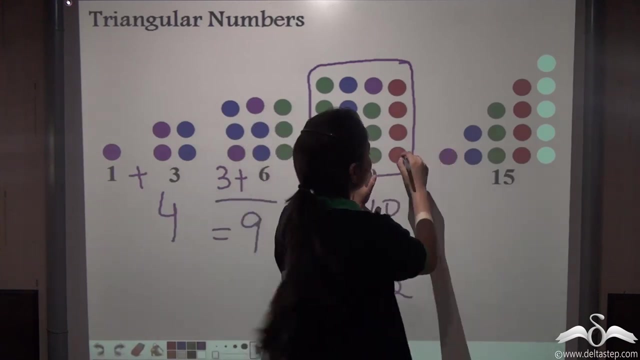 Now again, let us check the other ones also. Rotate this again, See what do you get: Again a perfect square. So adding 6 with 10 gives me 16. That is a perfect square of 4.. Similarly, adding 10 with 15.. 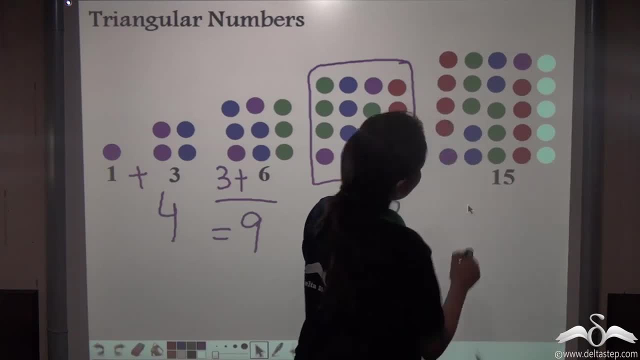 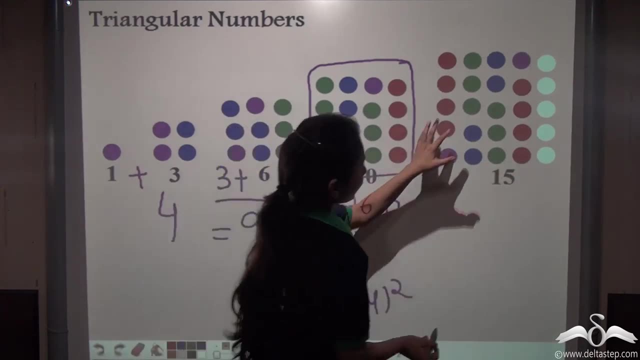 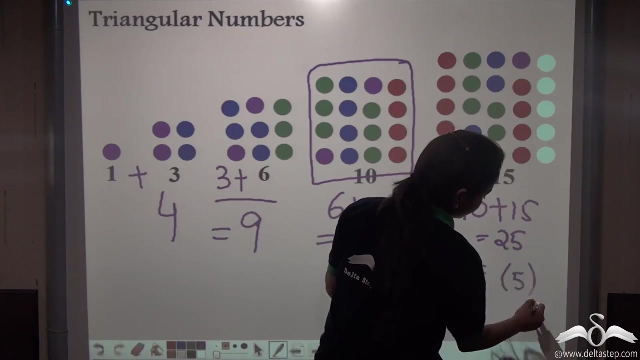 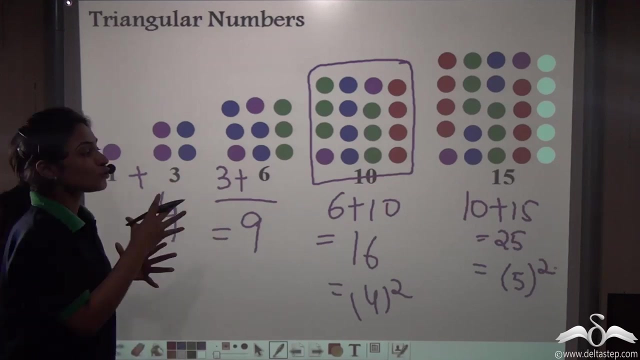 We are completing this square. See, it is a perfect square. So adding 10 with 15 gives me 25, which is a perfect square of 5.. So this is how triangular numbers they any two consecutive triangular numbers, they combine to form perfect squares. 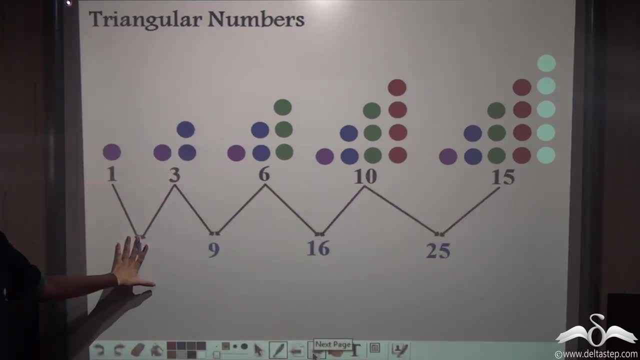 So you can see, 1 plus 3 gives us 4,, 3 plus 6 gives us 9,, 6 plus 10,, 16,, 10 plus 15,, 25, and they are all perfect squares. So this is a very interesting fact about the triangular numbers. 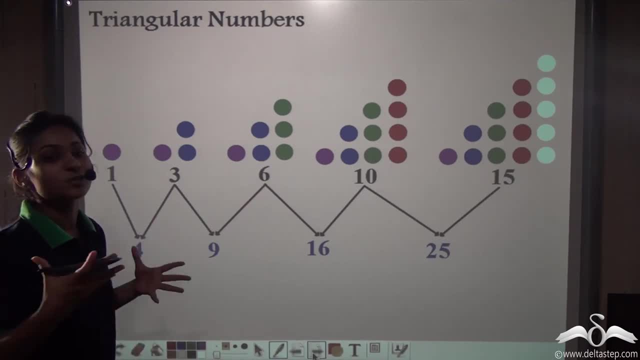 which, when any two consecutive triangular numbers are added, give us perfect squares. Thank you,